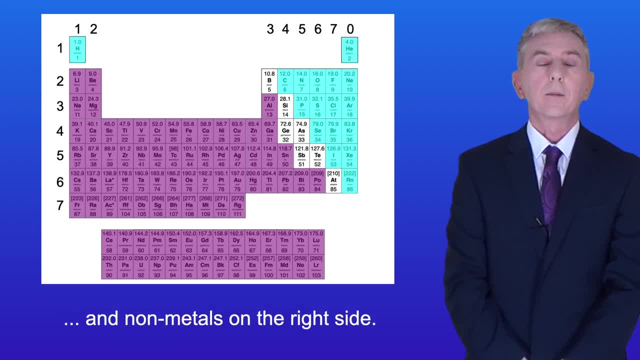 metals on the left side and nonmetals on the right side. Between the metals and nonmetals we find the metalloids, which are also called the semimetals. Metalloids have some properties of metals and other properties of nonmetals. In these two videos we're going to look at 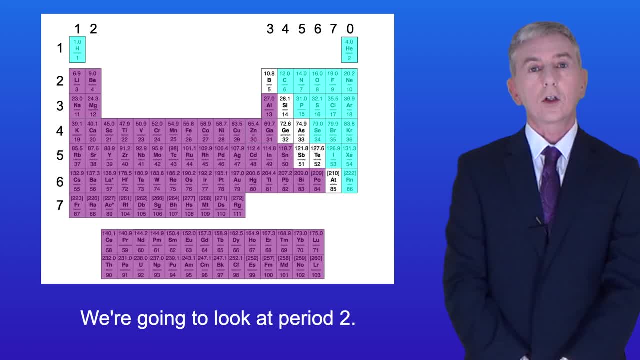 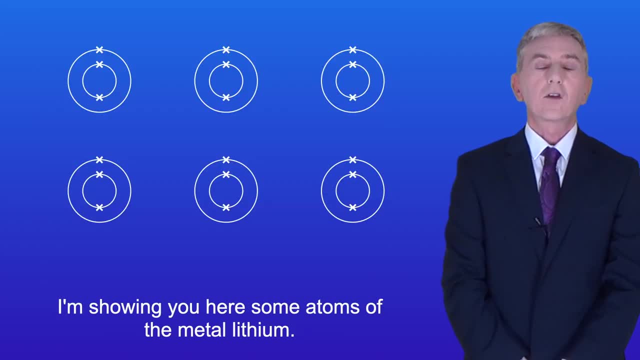 periodicity and structure. in the periodic table On the left of period two we have the metals lithium and beryllium. I'm showing you here some atoms of the metal lithium. Lithium atoms have three protons in their nucleus: Lithium. 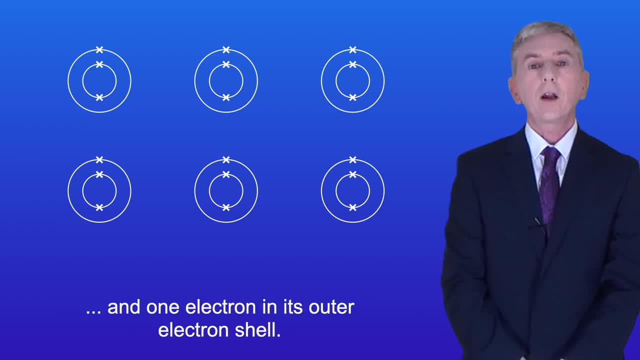 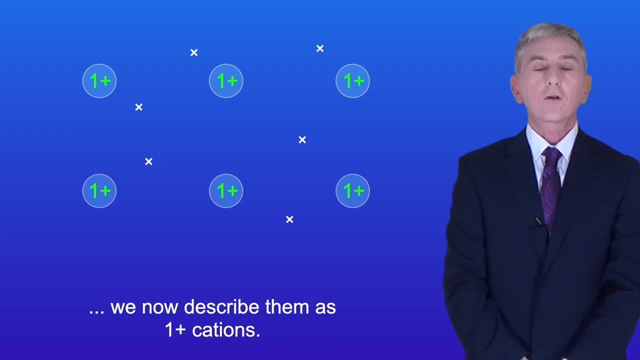 also has two electrons in its first electron shell and one electron in its outer electron shell. Now, in metals, the electrons in the outer shell are delocalized, In other words, they're shared like this: Because the lithium atoms have donated their outer electron, we now describe them as one-positive. 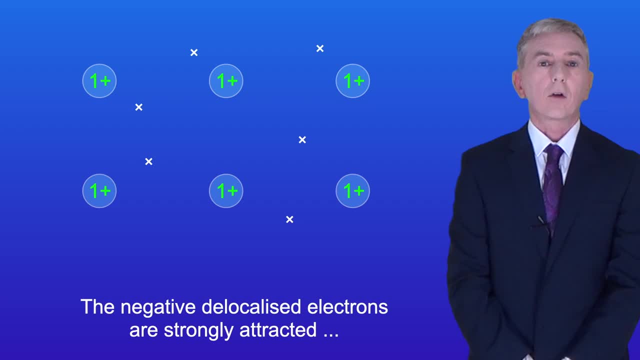 cations. The negative delocalized electrons are strongly attracted to the positive cations by electrostatic attraction. Scientists call this electrostatic attraction metallic bonding, And the overall structure of the metal is referred to as a giant metallic lattice. Now there are a couple of key features of the giant metallic lattice that you need to. 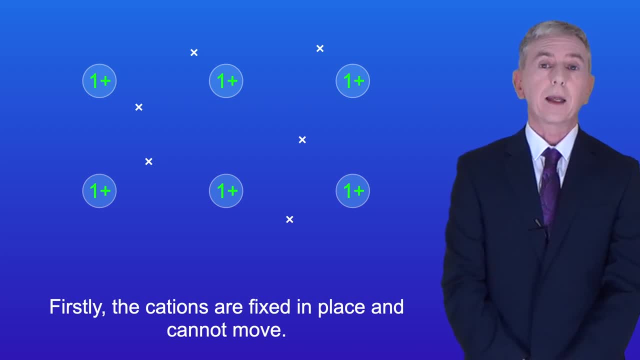 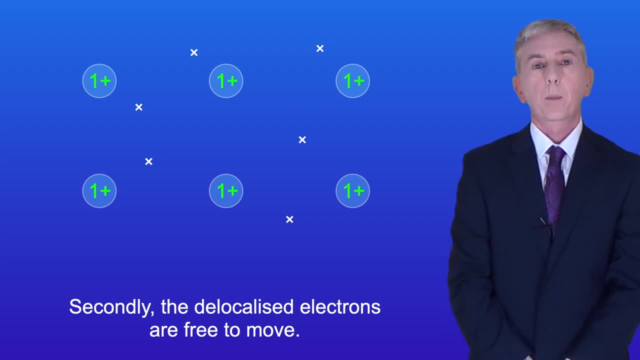 Secondly, the delocalized electrons are free to move. Now, because the delocalized electrons can move freely, this explains an important property of metals. Metals are good conducts of electricity when they're both solids or liquids. I'm now showing a voltage across the metal. As you can see, the delocalized electrons have. 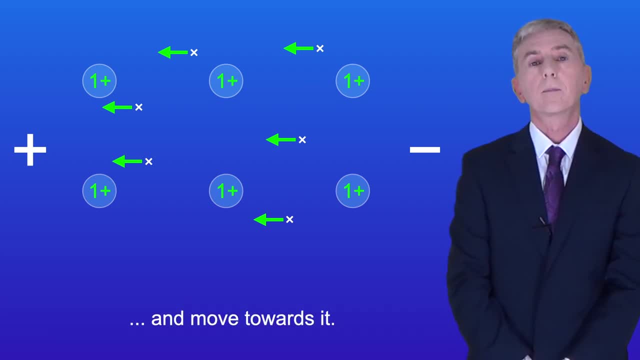 attracted towards the positive pole and moved towards it. In this case, the delocalized electrons have attracted to the positive pole and moved towards it. Delocalized electrons are acting as mobile charge carriers, enabling metals to conduct electricity. Now, another property of metals is that most metals have relatively high melting and boiling. 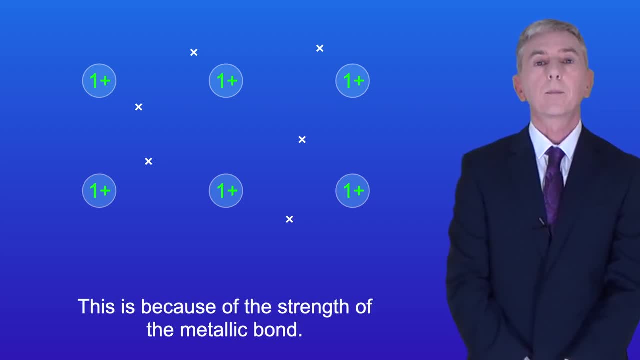 points, and this is because of the strength of the metallic bond. Remember that the delocalized electrons have a strong electrostatic attraction to the cations. It takes a lot of energy to overcome this attraction and this means that metals generally have high melting and boiling points.